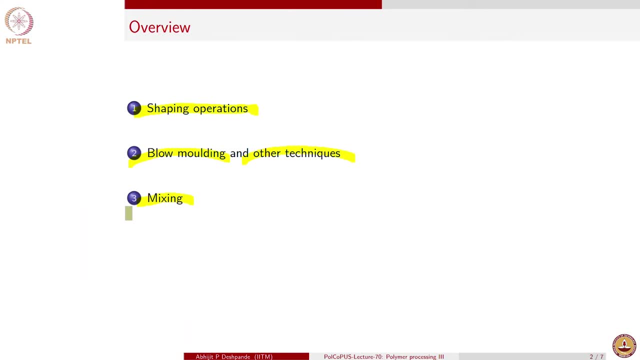 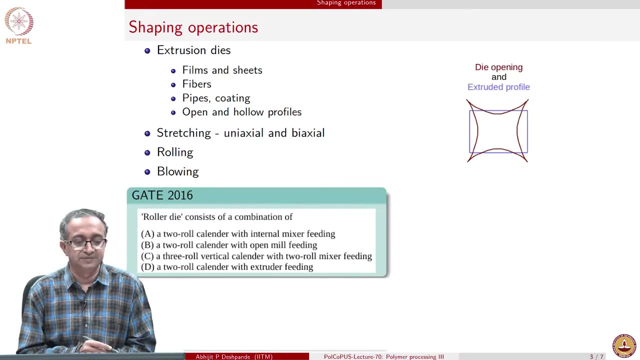 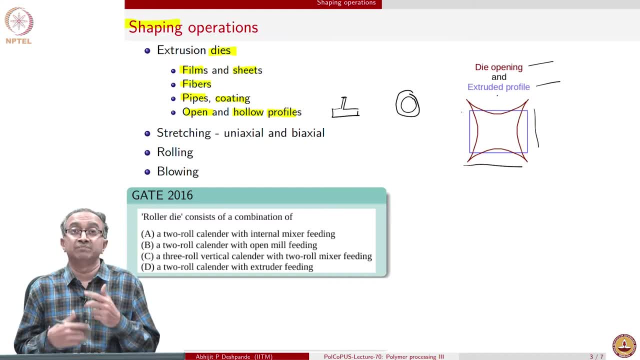 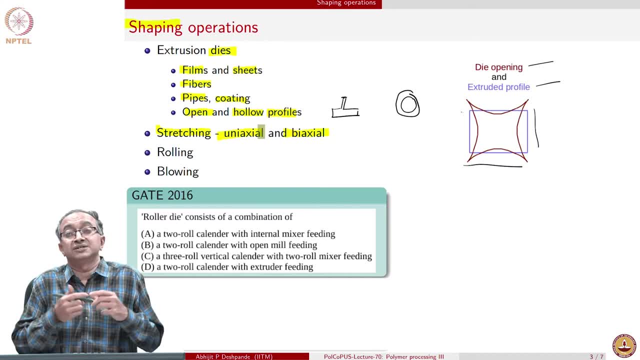 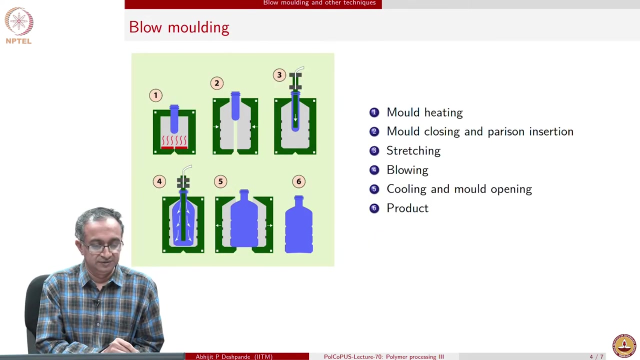 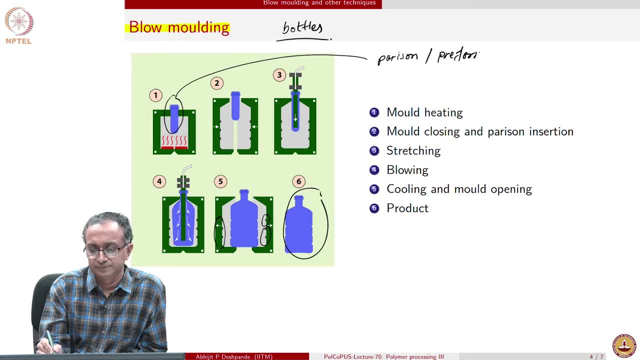 pre form. So there are 2 ways in which this blow molding operations is done. some time you extrude this at the same time blowing can happen, and then you can make the part, or you can injection mold this And then just put it here and then do the blow molding. 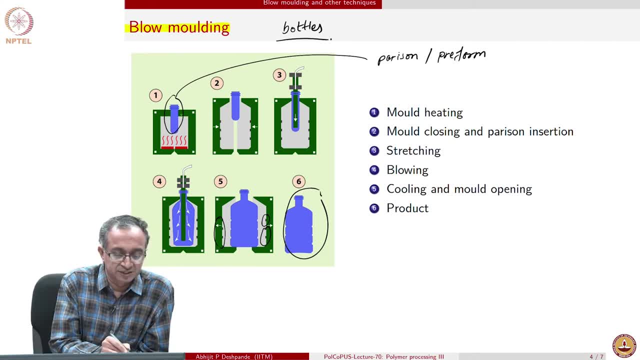 operation. So, for example, here this is been injection molded and now what you do is you close the mold and heating is done so that this blue polymeric material can deform, and then what you do is you inject a rod. So this is called. 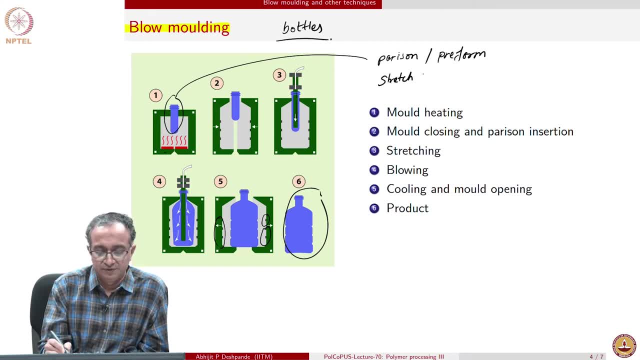 stretch, blow molding So you stretch, so that polymer molecules get oriented. You must have noticed that some bottles are extremely thin and still they can withstand the amount of water filling. that happens and the load that it is supposed to carry. and partly this is because 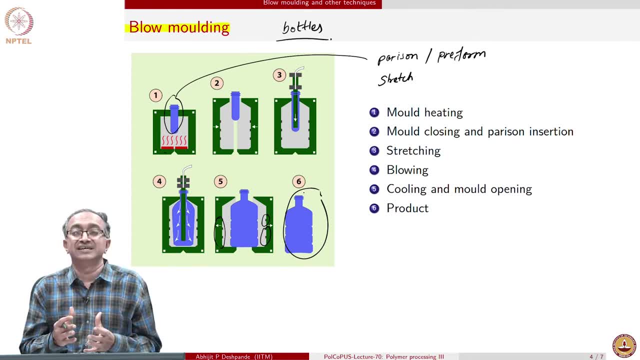 the orientation has been manipulated by doing stretching and through these reinforcements, these shapes, So that with least amount of material you can have requisite performance in terms of holding the water and not breaking. So stretching or stretch blow molding, involves stretching, Stretching the polymeric material initially, so that molecules get oriented along the direction. 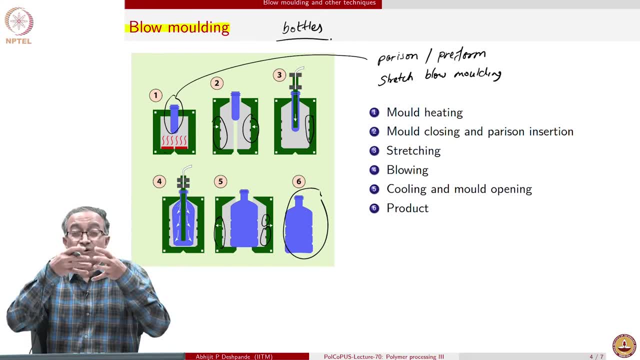 and then blowing. So the fourth stage is where now the gases are blown into the material and since mold is closed, what happens is this material will go and then conform to the mold surface, And once the conformation happens, then you can immediately start cooling and or stop heating. 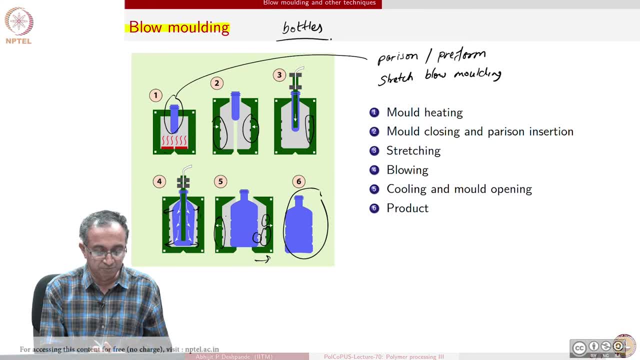 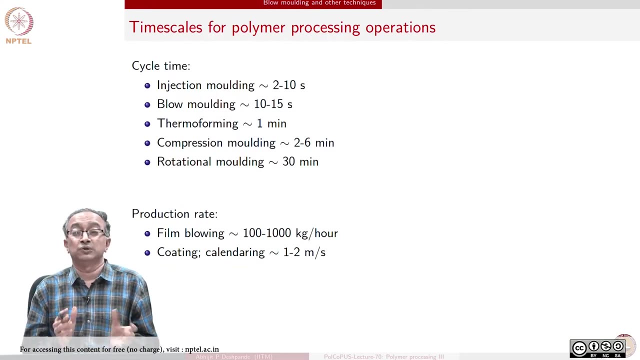 and then separate the mold So you can see that these parts will be based on whatever is the mold features and then you can get the product which is. and all of this process can happen very quickly. And just to give you how quick or slow the process is, injection molded cycle time is less than 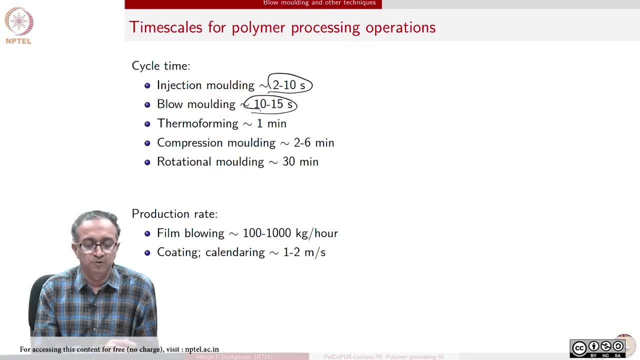 a second, less than 10 seconds, while blow molding is also not very slow- 10 to 15 seconds- one can get a bottle out. Now you can see why there are so many different processes, So many different plastic bottle products out there, compared to glass or ceramic container making. 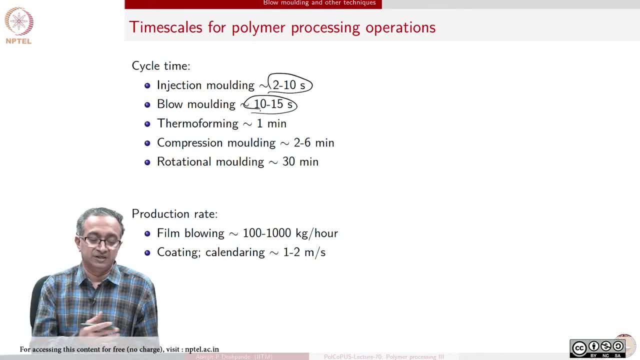 these are extremely inexpensive operations because you can achieve volumes very quickly. Very large amount of bottles can be manufactured in very short amount of time. Thermoforming, which is also a quicker technique, where we shapes are largely flat or slightly curved and it is like a stamping operation which is used in 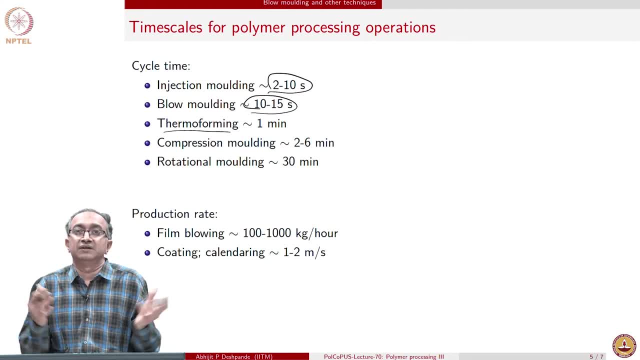 melt And so thermoforming. the shaping is done between two platens and therefore the shape cannot be very complex, but again, it takes just about a minute to complete the operation. Compression molding, on the other hand, can have more complex operation, but it takes more amount of time, And many of these cases there are finer features, for example, 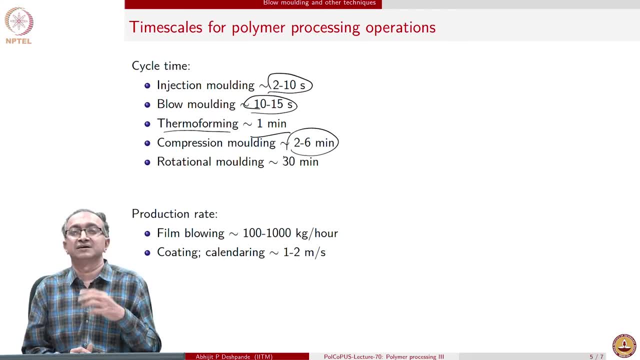 whenever we do we are doing these operations, it is possible that gases or air can get entrapped, Which will lead to voids. So in all of these cases we will have to manipulate the pressurization closing opening in such a way to minimize entrapment of voids or the 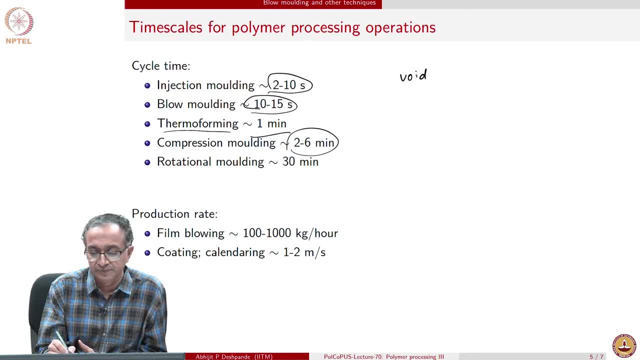 void generation. So void generation is a very important defect during polymer processing and this needs to be minimized. In compression molding, for example, this can be done sometimes by doing what is called breathing, So we can close the compression mold, then open it little bit and again close it to allow the gases or voids which are there to escape. 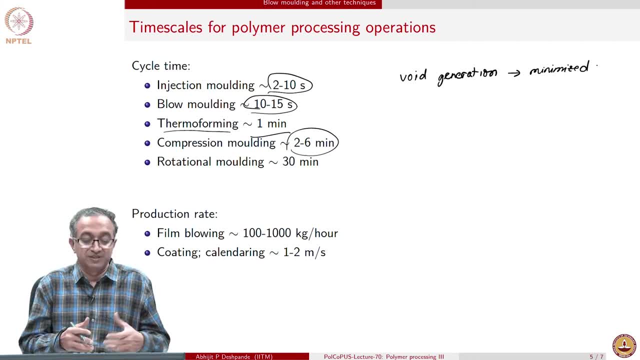 And so that is why it is called a breathing operation. We hope that the polymer will exhale the voids out. On the other hand, the tanks which are made using polyethylene, quite often water storage tanks. that takes about a 30 minute, So through rotation. 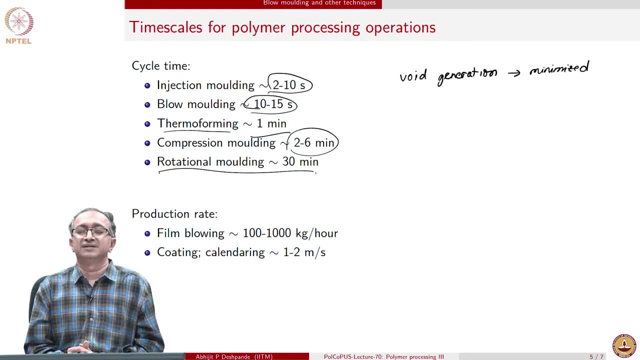 rotational molding, basically the thickness of the tank is made, And these are quite thick tanks as opposed to the bottles or other thinner blow molding bottles or blow film blowing thin films. Rotational molded tanks are quite thick. These are supposed to hold thousands and thousands. 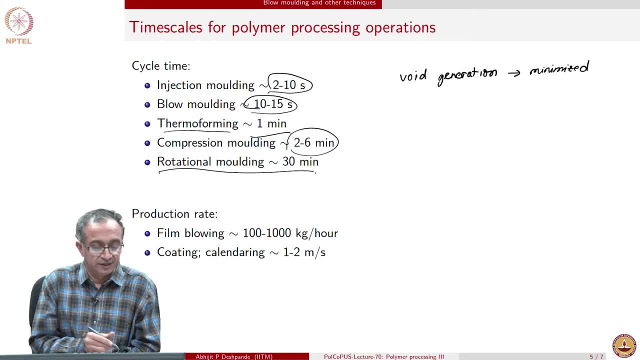 liters of water or other substances. In the case of continuous production units, you can see the mind boggling amount of material that can be produced. In one hour we can make 1 ton of film And remember these are very thin films, So this is an extremely large amount of polymeric films. 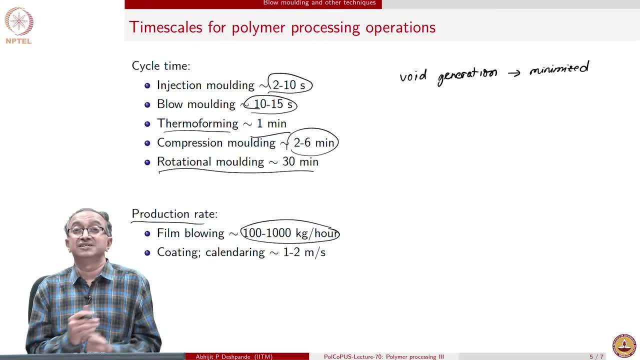 that can be made, And therefore you should not be surprised that why these films are so ubiquitous. And as polymer scientists and engineers, it is now our responsibility to figure out sustainable ways of doing this. Coating calendaring can also be reasonably rapid, where in a second we can process. 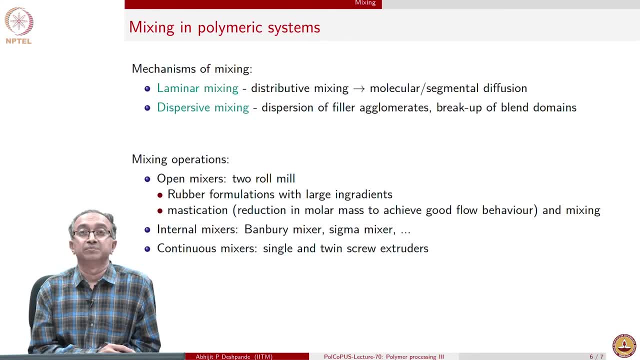 a couple of meters of material. So in all of this, mixing is also equally important, And mechanisms of mixing in case of polymers are quite different compared to mixing in, let us say, oil or water or air and things like that, And that is because of the presence of turbulence. 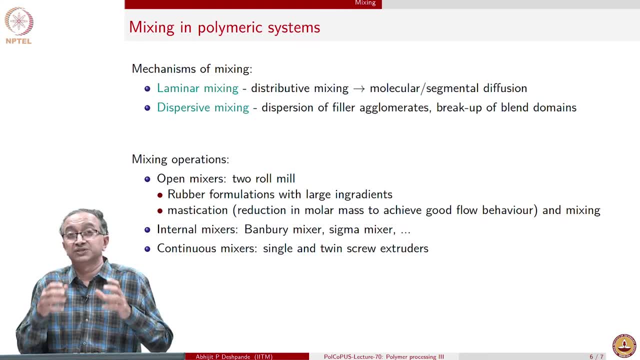 Because, in case of polymers, the viscosity is extremely high, turbulence is not observed And because turbulence implies that you know there are small eddies getting formed, broken, and there are lots of fluctuations in velocity and pressure at each and every point. 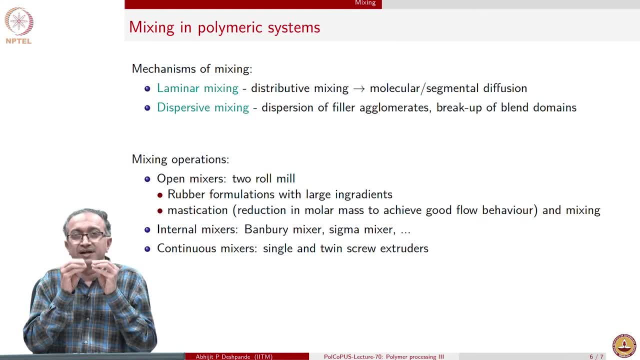 mixing is actually quite fast And once these eddies get broken down to very small level there can be quickly molecular mixing which is based on diffusion. But in case of polymer there is only laminar flow possible, which means one sheet of polymer moves, another sheet of polymer moves next to it, And these two 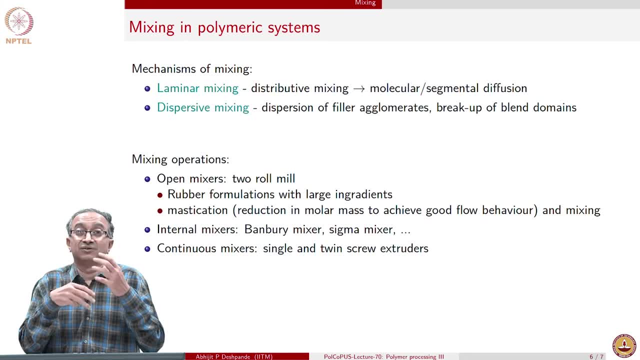 moving at slightly different rate. So mixing can only happen predominantly because of molecular and segmental motions. So laminar mixing, some amount of mixing happens, but eventually the rate determining step is molecular, segmental diffusion. We can we have, of course, if we have some fillers or if we have blend domains, then we can also have. 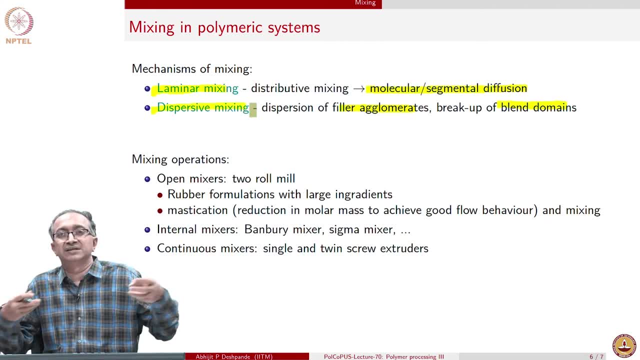 a dispersive mixing where the agglomerates can get broken and then they can come together and so on, Or the blend domains can get broken, So there is a distribution or dispersion of these fillers and domains through which again mixing can happen. 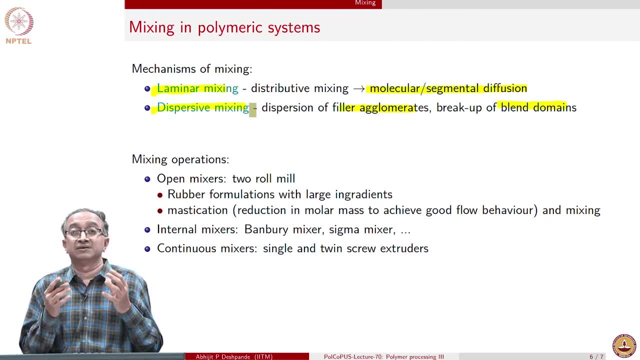 And generally these mixing operations- given that macromolecular mixing is very important in the end to get the final performance- are done using several different types of operations. If we have basically rolls as part of mixing, so we can pass the material through a set of rollers, 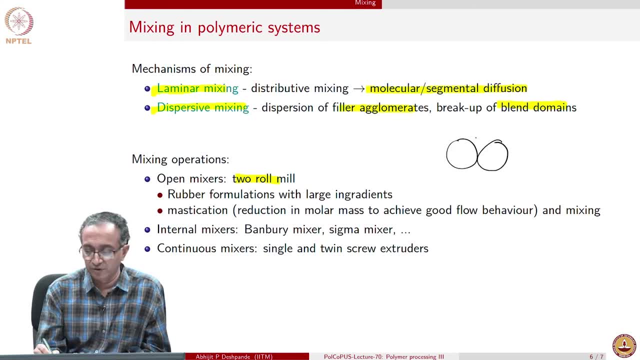 So there is a narrow opening through which we can. So we have the polymer, polymeric material, and then we can force it by having these two rollers rotate And then we get the material out, because now we are forcing it through the narrow opening and we are shearing the material and 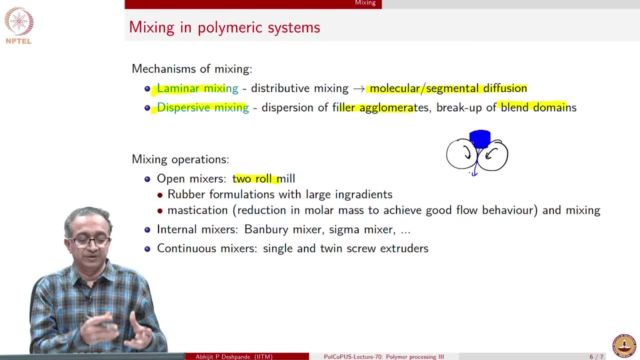 mixing will also happen, But again this will be laminar mixing And dispersive mixing, because latex are mixed this way. it is a multi-phase system, So therefore particles can come together, particles can separate, And so it will have a combination. 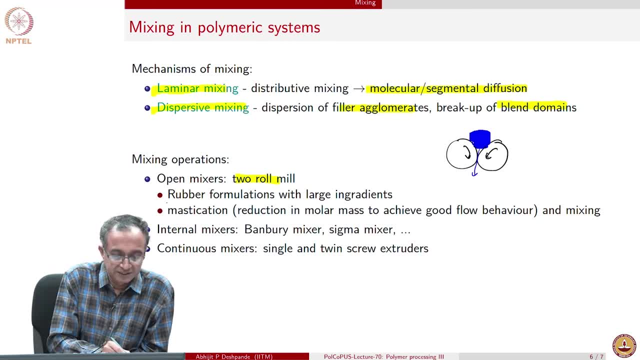 of laminar and dispersive mixing. So rubber formulations, for example, are processed this way because there are large number of ingredients which have to be mixed. We can also use this to achieve a good molar mass, because chain scission and other processes 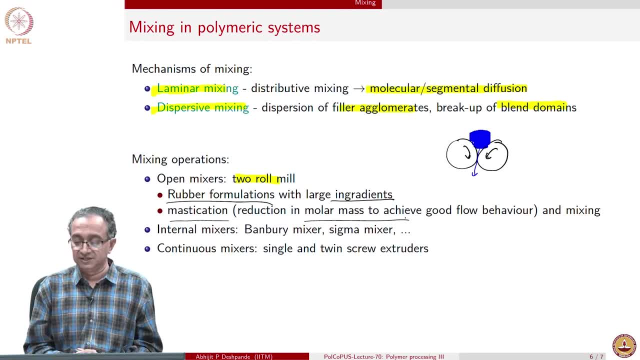 can happen because of high rates of shear which are generated in such processes. So we have both mixing as well as mastication. We have, of course, internal mixer, in which case we have a vessel in which a specific impeller or a blade is put, and then this is rotated. 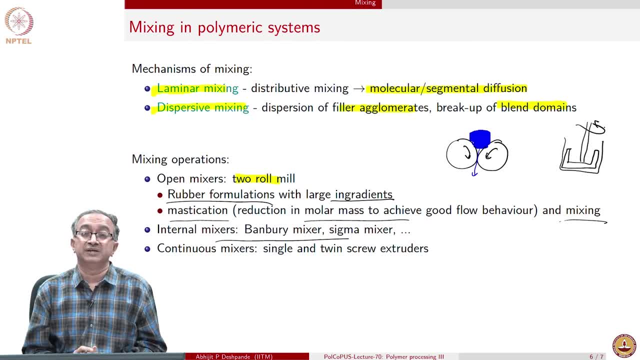 And again, because of very high viscosity of polymeric materials, the mixer and the blades are very different design compared to mixing in case Of low viscosity fluids, And so we have something called a sigma mixer and a Banbury mixer, And crucial aspect in each of these is to have this impeller design. 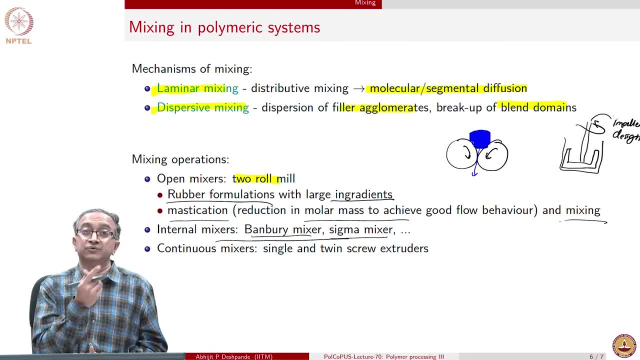 It is very possible, because of very high viscosity, that when we are doing this impelling action or stirring action, lot of material does not get stirred at all. So you have to have an impeller design which ensures that everywhere mixing happens At the same time. this cannot be done very fast because the viscosities are extremely.